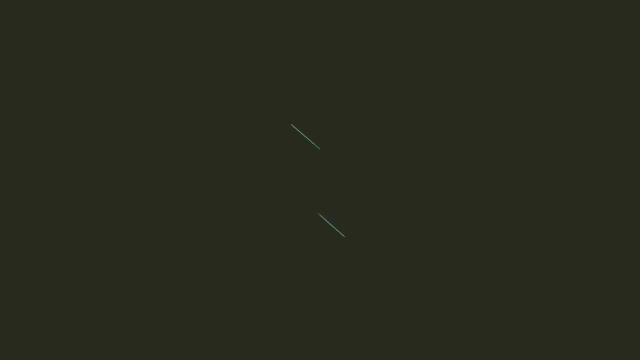 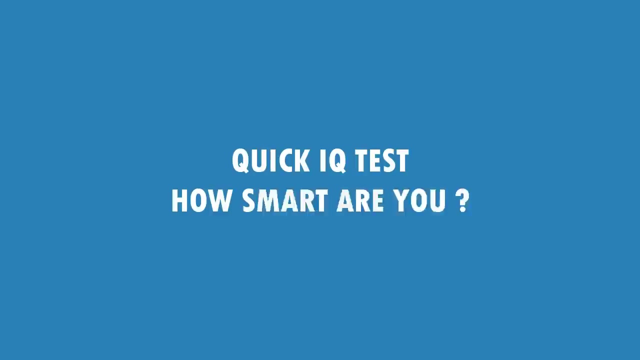 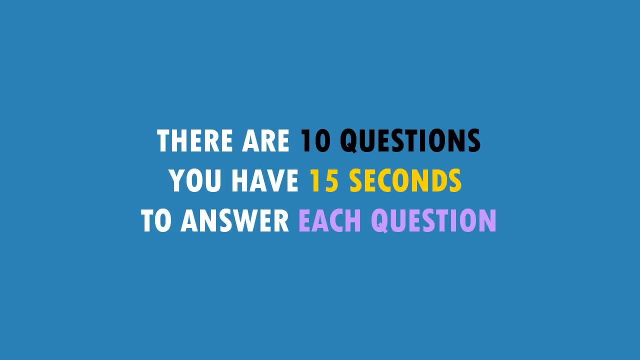 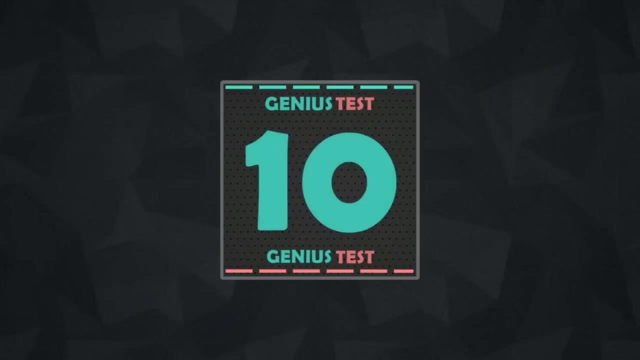 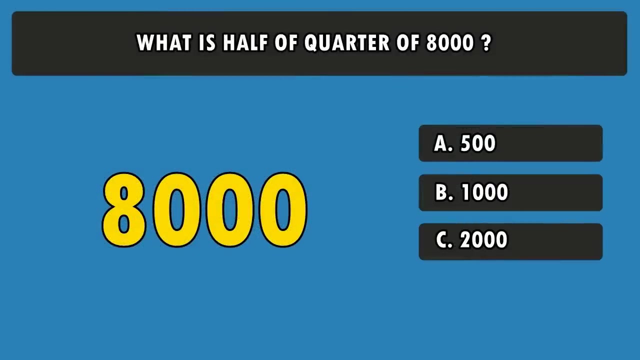 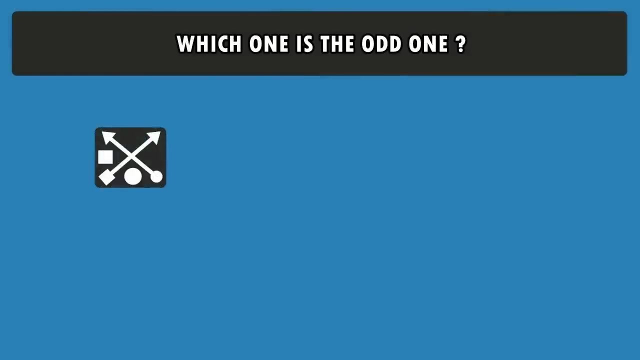 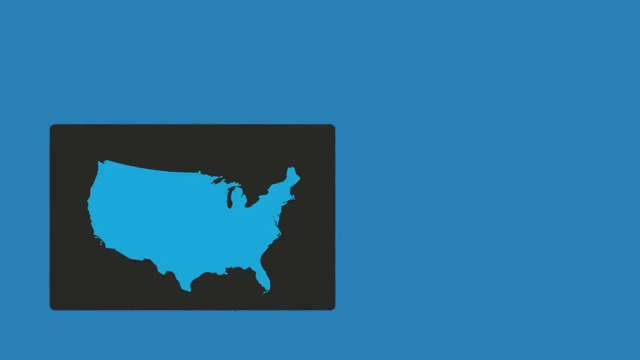 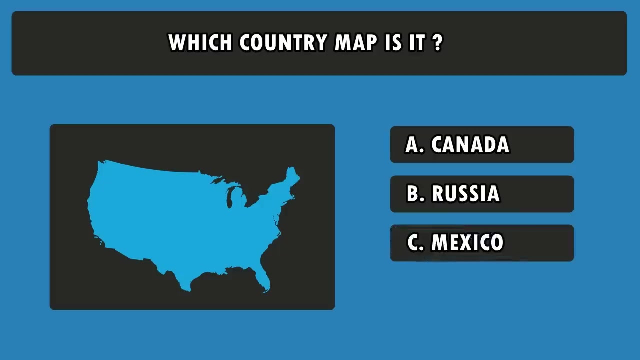 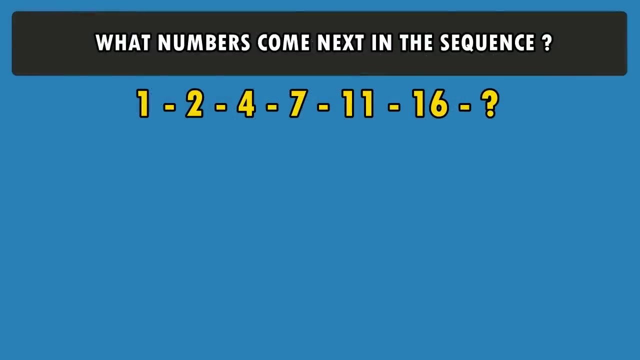 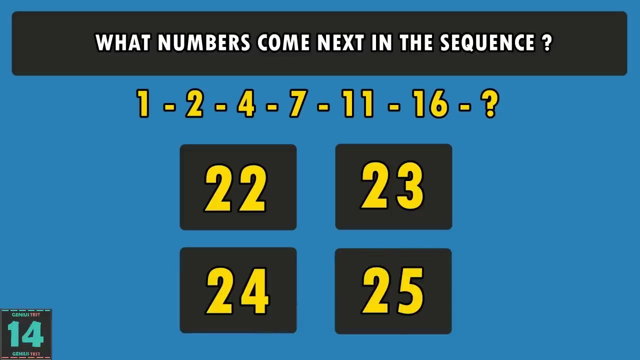 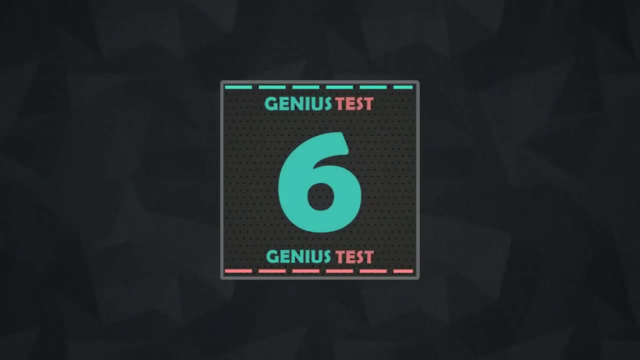 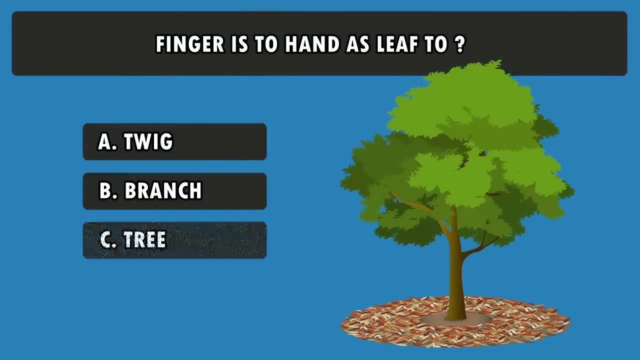 Thank you for watching. Number 10, Number 9, Number 8, Number 7, Number 10, Number 11, Number 12, Number 13, Number 15, Number 16, Number 18, Number 19, Number 20, Number 21, Number 22, Number five.